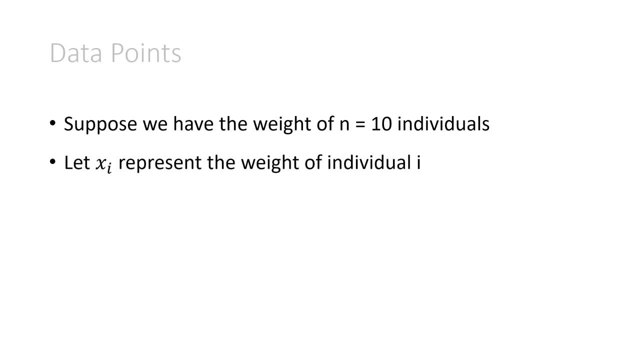 n equals 10 individuals. Let xi represent the weight of individual i, Then x1 is the weight of individual 1.. x2 is the weight of individual 2, and so on. We'd have this all the way up until xn, and since n is equal to 10 in this example, we'd have it all the way up until x10. 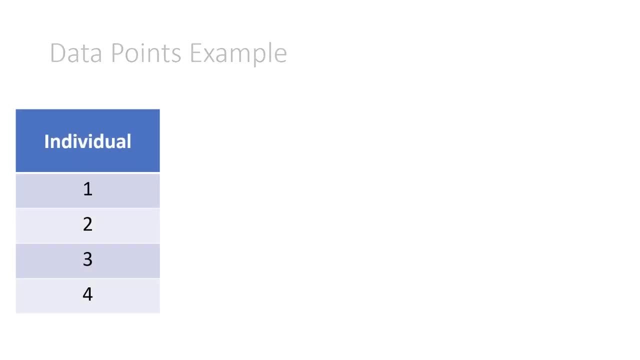 Okay, let's look at an example. We have four individuals, so that's setting n equal to 4.. You can set n equal to any positive integer and this should work, And we have their weight in kilograms. The first individual has a weight of 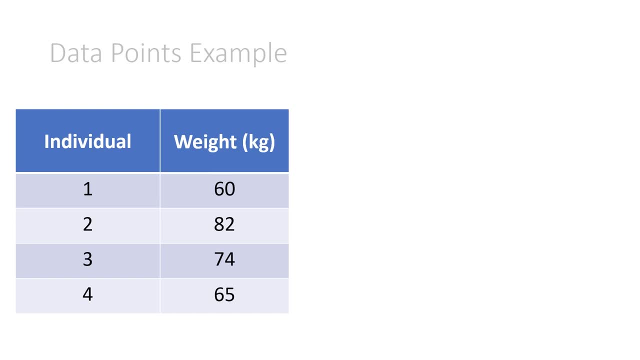 60 kilograms, second is 82,, third is 74, and fourth is 65. So, using our notation, let xi represent the weight of individual i. Then we know that x1 is equal to 60,, x2 is 82,, x3 is 74,. 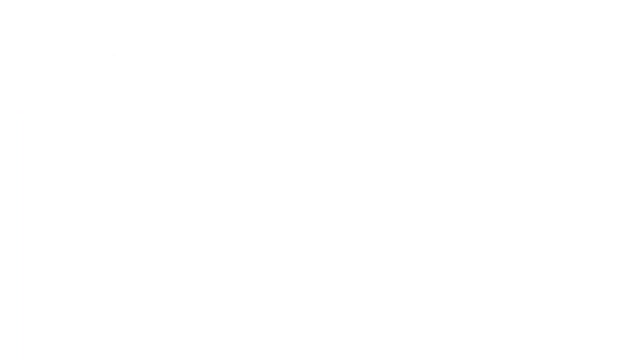 and x4 is 65.. Now, that was one-dimensional data. We only had their weight, But let's look at two-dimensional data points and we'll also get their height. Suppose we have the weight and height of n equals 10 individuals. Now we have to have a second. 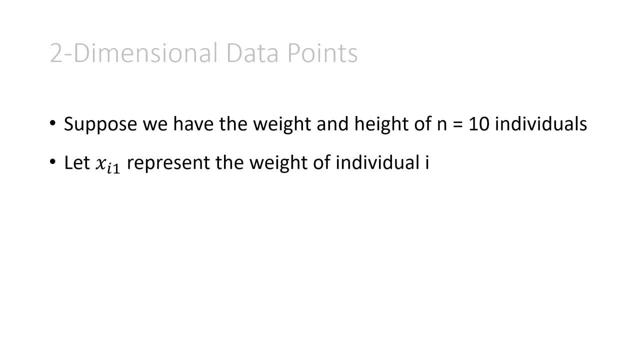 subscript. We'll let xi1 represent the weight of individual i and let xi2 represent the height of individual i. Then x11 is the weight of individual 1, because the first subscript is 1,, so that means individual 1, and the second subscript is also 1,, which means their weight. 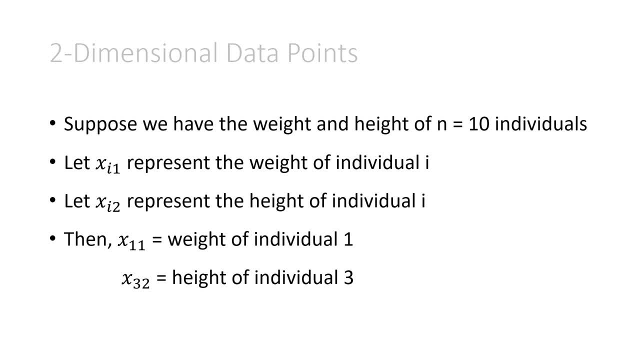 And so on. You could have x11,, x12,, x21, x22, up until xn1 and xn2.. That might have sounded confusing. Don't really worry about it. Okay, let's look at a similar example to before. 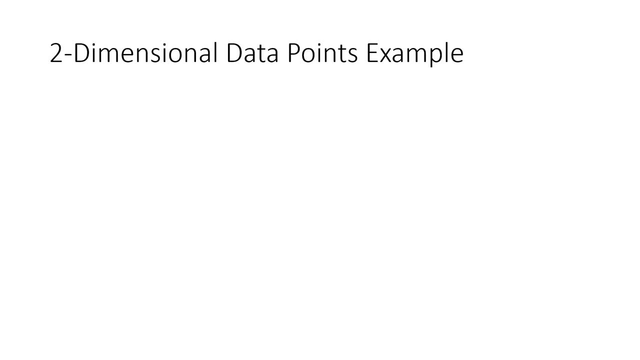 So a two-dimensional data points example. Two-dimensional because we have both their weight and their height. That's two dimensions. We have each of their weights in kilograms- same people as before, and we'll mark that as column 1, which will be useful to mark the second subscript- And we also have their height in kilograms. 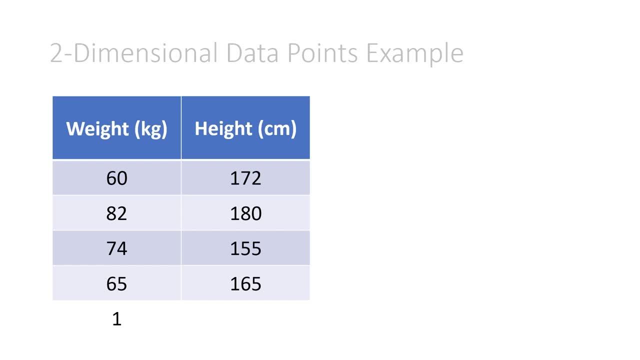 The first has a weight of 60 kilograms and a height of 172 centimeters and so on, And we'll mark the height column as column 2.. And just a reminder, the first row represents the first individual, 2,, 3, and 4.. So again, n is equal to 4 in this example. 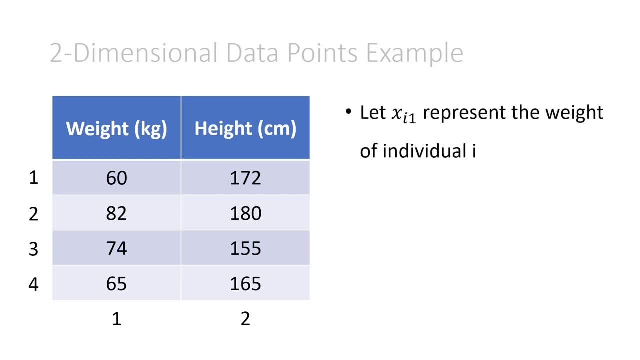 Keeping our same notation, we'll let xi1 represent the weight of individual i, Let xi2 represent the height of individual i. So x11 is equal to 60.. You can think about this. as for the first subscript, you look up the row and the second subscript, you look up the column. 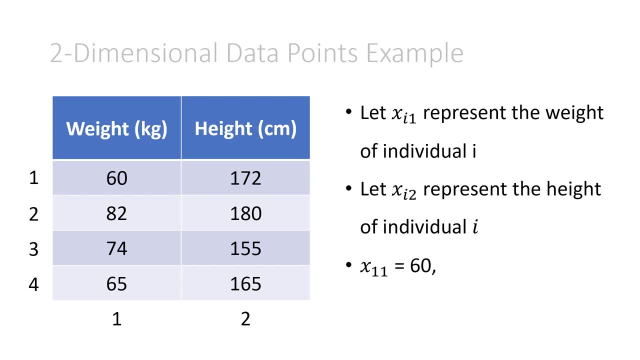 So xi1 goes to the weight of the first individual, which is 60 kilograms, and x32 is 155.. So the third row and the second column, that means a height of 155 centimeters, And you could do this for the other ones as well. 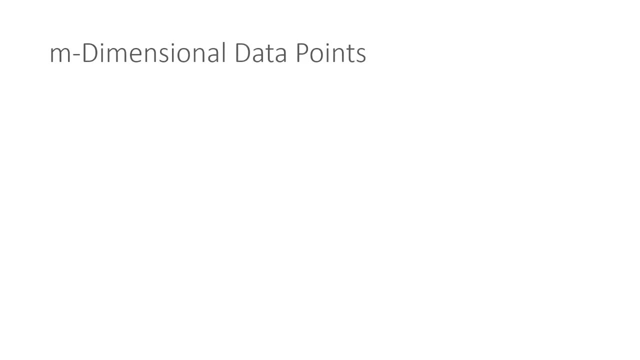 Okay, that was two dimensions, which is better, but really we want m-dimensional data points, We want to know an arbitrary amount of attributes, an arbitrary amount of information about n. So, firstly, suppose we have m many attributes, for n equals 10 individuals. 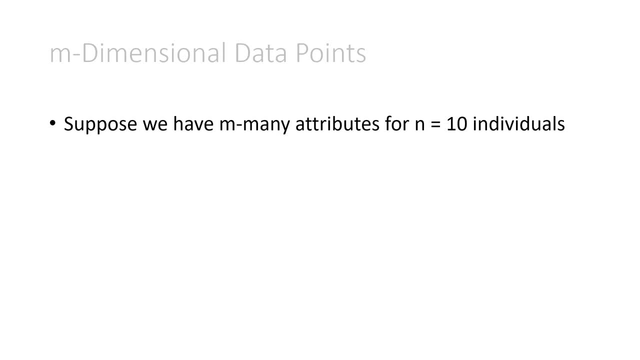 As long as m is a positive integer, like 1,, 2,, 3, and so on, then the math will still work out. Let xij represent the jth attribute of the ith individual, Then x43 is the third attribute of the fourth individual. 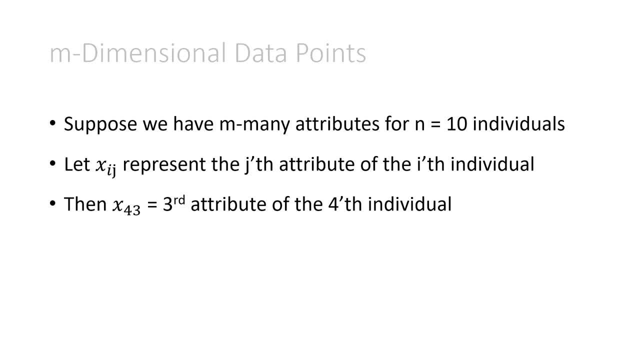 Again, the first subscript still looks up the individual, So it's the fourth individual, so the first subscript is 4, and it's the third attribute, so the second subscript is a 3.. Now let's look at an example of these m-dimensional data points. 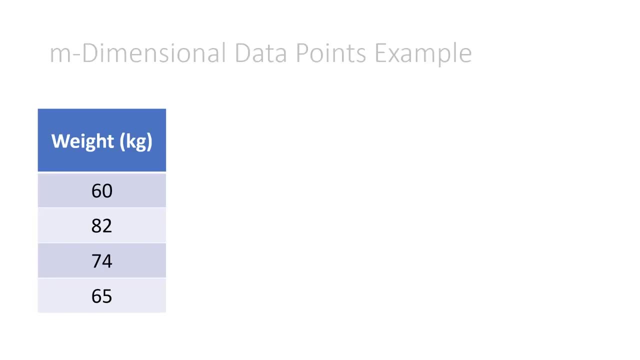 We know m different things about each individual. We'll still use their weight. so we have n equals 4 individuals. We have each of their 4 weights. We'll mark that as column 1.. We also know their height. the same column as before. 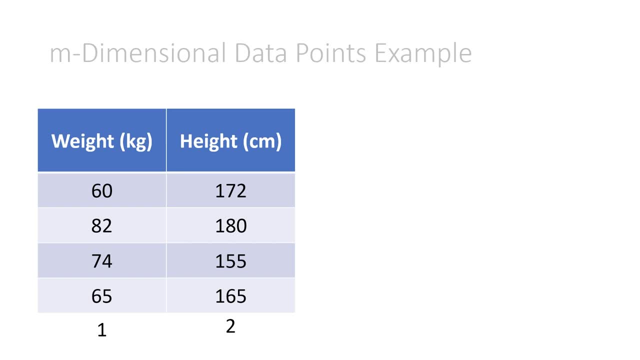 Mark that as column 2.. And in this example we'll set m equal to 3.. So this is the last column we'll have. We'll have what country they're from. The first individual is from Canada, Second is from India. 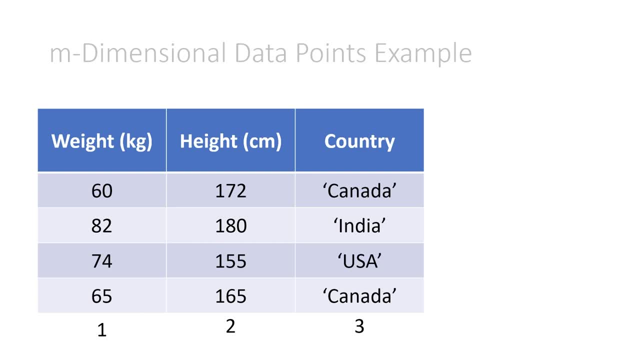 Third is from the USA And again the last is from Canada as well. And again, a reminder of the rows: The first row represents the first individual, which has a weight of 60 kilograms, a height of 172 centimeters, and they're from Canada. 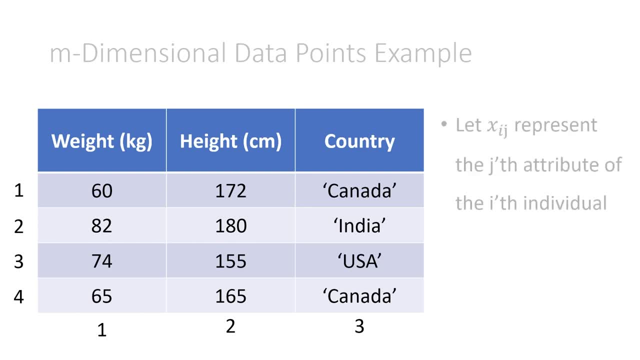 Individual 2,, 3, and 4.. Now, keeping with our same notation, let xij represent the jth attribute of the ith individual. The first attribute is the weight, the second is the height and the third is the country. 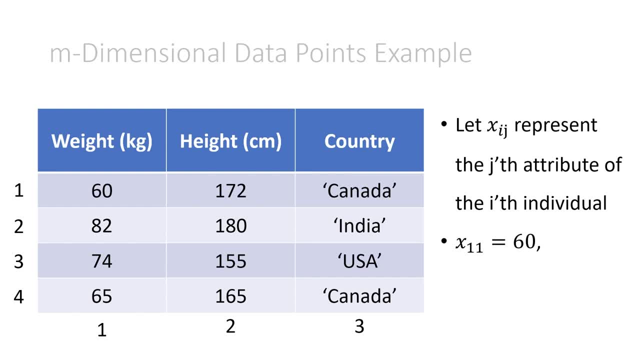 So then, x11 is 60.. That's still looking up the first row and the first column, which is 60 kilograms. x42 is 165.. So the fourth row and the second column marks 165.. And so on, And so on. 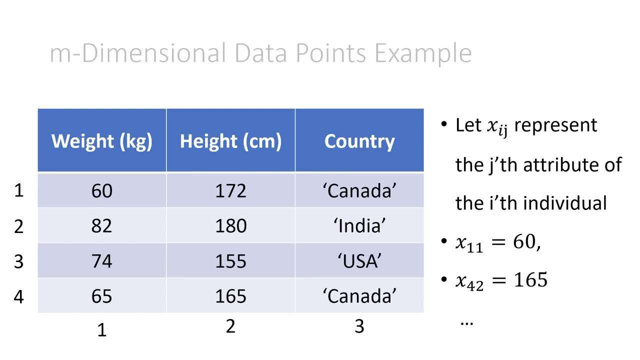 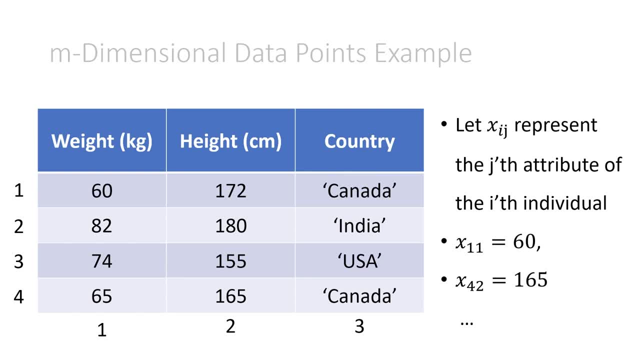 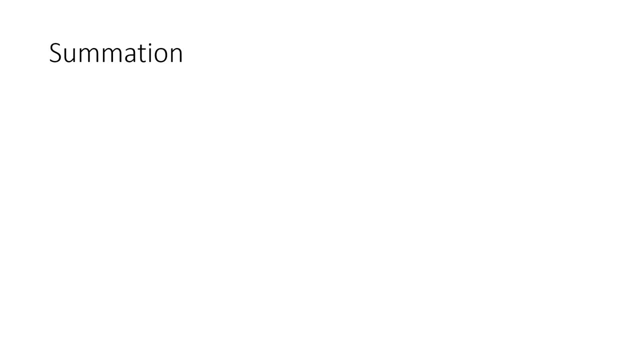 they'd call this a matrix. Now let's look at some common mathematical operations that we could perform on this table. Firstly, summation: Let's look at the notation. for that We often need to perform a matrix. We can perform summations, which is just addition, adding a bunch of things together. 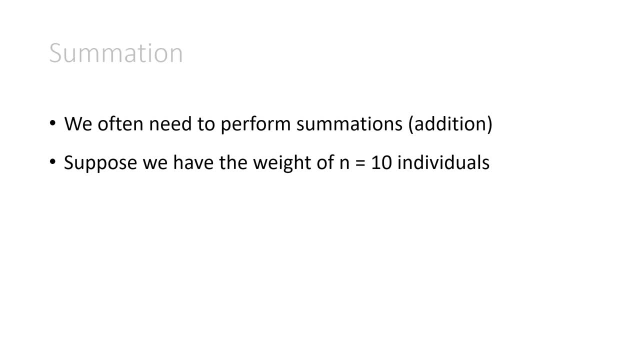 Suppose we have the weight of the n equals 10 individuals, and again we'll let xi represent the weight of individual i. back to what we had at the beginning. This new notation reads as the sum, as i goes from 1 to n, of xi, and that's defined as. 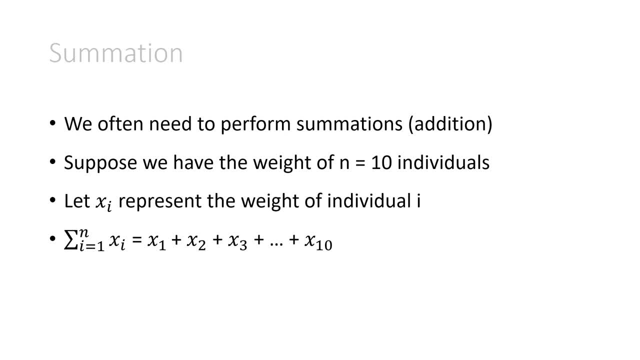 x1 plus x2 plus x3, all the way up until x10.. The sum goes over all of the xij from i goes from 1 to n, so whatever n is equal to, since n is 10 in this example, we're adding x1 plus x2, all the way up until x10. 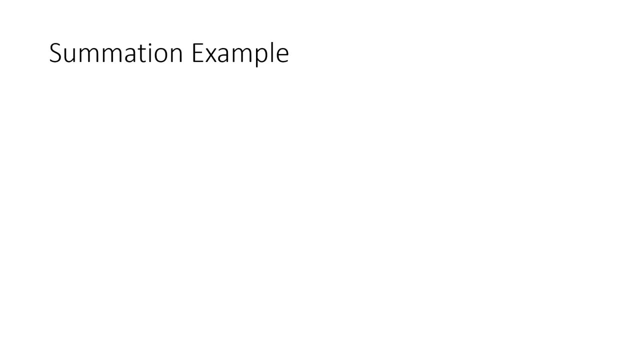 Again, let's look at an example, So a summation example. Let's have the individuals, four weights. mark it 1,, 2,, 3, and 4.. Let xi represent the weight of individual i. Then in this case the sum, as i goes from 1 to n, is equal toouts per x. The i equals one. down. then comes over the x and the sum of x, again of numbers, i equals x2 and x3 plus x3 minus x3.. The first sum is an egalism sum, which so sets the sum as i goes from 1 to n, as i goes from. 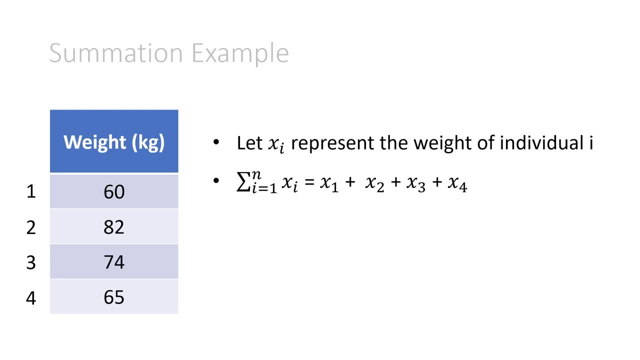 one to n. The sum over all the xi's- from i goes from 1 to n- of xi is x1 plus x2 plus x3 plus x4. Since n is equal to 4, it stops at 4.. And if you were to look, 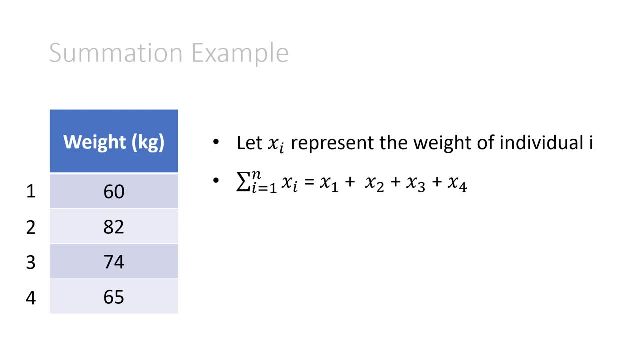 up what x1 and x2 and x3 and x4 is. it's 60 plus 82 plus 74 plus 65. That's just the sum of all of the weights and that is equal to 281.. It's just saying that the sum of all of the weights in this 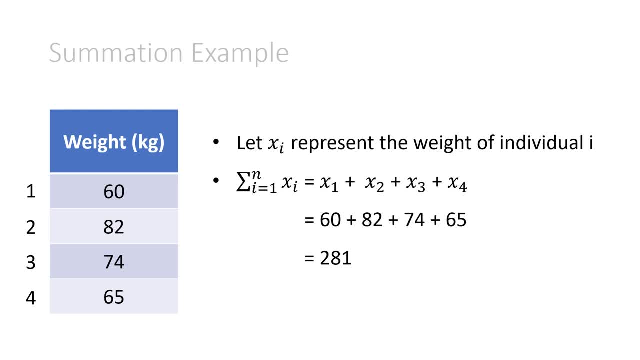 case is equal to 281.. This might not seem useful, but the notation on the left-hand side of the equals sign is used all over the place in mathematics. It's a nice short form for a sum. Now something very similar that comes up a little less often, but still fairly often. 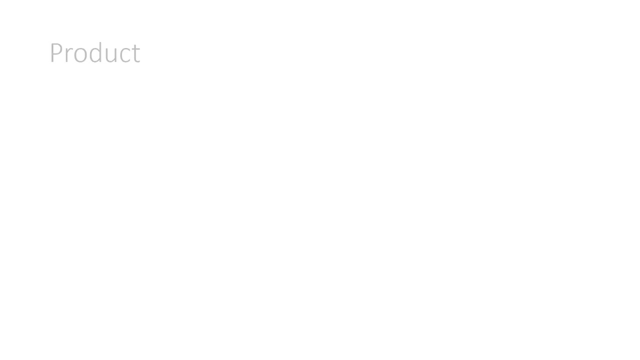 is the product. It's the same thing, but multiplying many things together We often need to perform products or just multiplication. Suppose we have the weight of the n equals 10 individual. We're going to multiply the product by the sum of all of the weights. 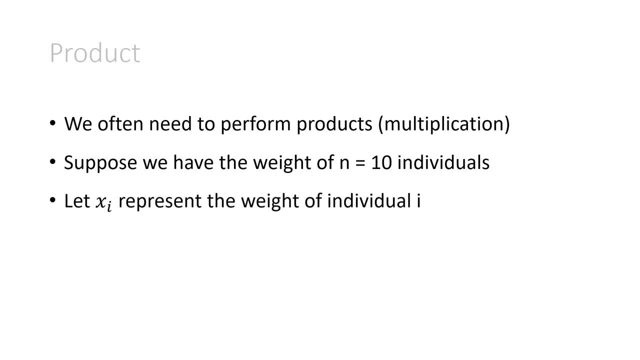 Let xi represent the weight of individual i, and now this new notation reads as: the product, as i goes from 1 to n of xi, is x1 times x2, times x3, times x4, all the way up until times xn. and since n is 10, it's times x10.. This is simply just the multiplication of all of the weights. 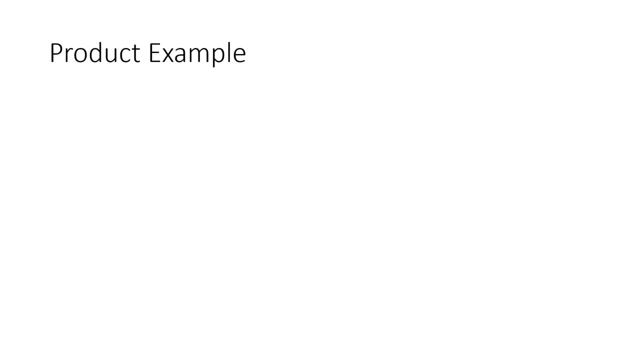 together. So let's look at an example, a product example. We have our four weights: 1,, 2,, 3, 4.. We let xi represent the weight of individual i and so the product, as i goes from 1 to n of xi. 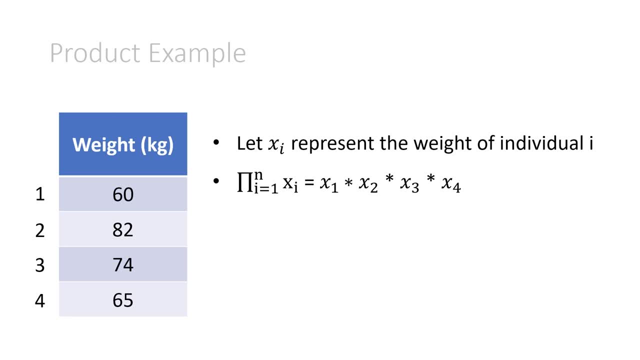 is all of them multiplied by each other, x1 times x2 times x3 times x4,, which is 60 times 82 times 74 times 65, and that mathematically is 23,665,200.. I totally worked that out in my head. 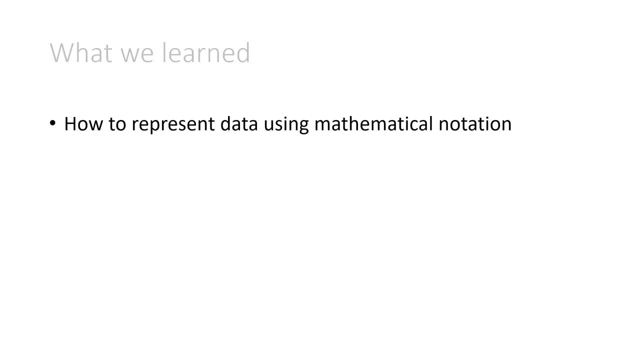 Okay, so what we learned? How to represent data using mathematical notation, How to store data in tables, And common operations such as summations and products. That's the end of this video.